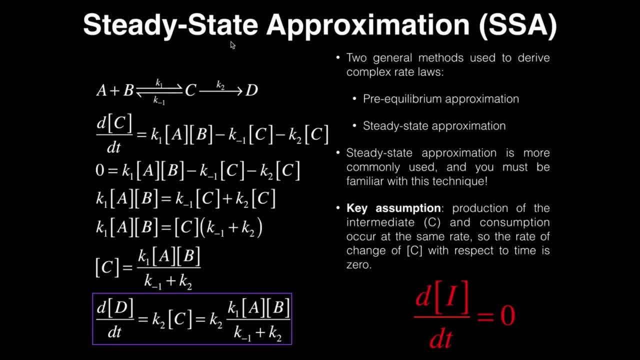 it pretty much is just the steady-state approximation, So this one is very important to understand. Alright, let's look at the equation right here. So I've got a chemical reaction. A plus B, these are my reactants or substrates. they're in equilibrium with species C and the forward. 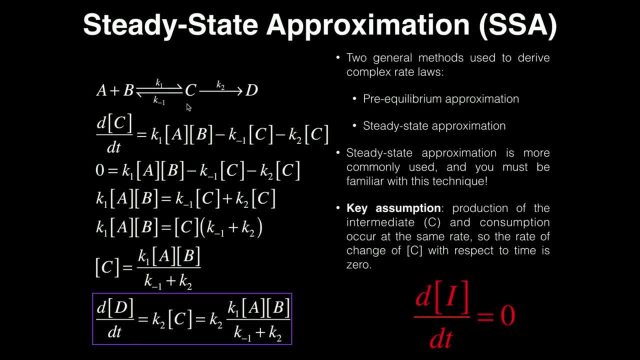 reaction of the equilibrium is K1,, the reverse is K-1, and then C can be consumed to form D, and that's expressed by this one-way rate, constant K2.. Alright, so in this reaction, C is what we call an intermediate, because it's being consumed by the 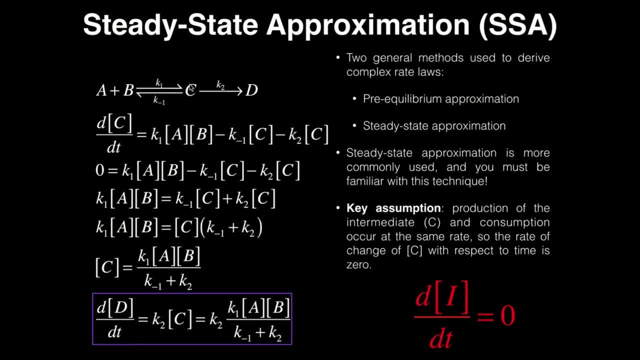 reaction of K2, but it's also being formed through the reaction of K1, and so C is going to be our intermediate here. Now, what is the steady-state approximation? This is an assumption, and it says that the rate of the formation of this intermediate, C, is 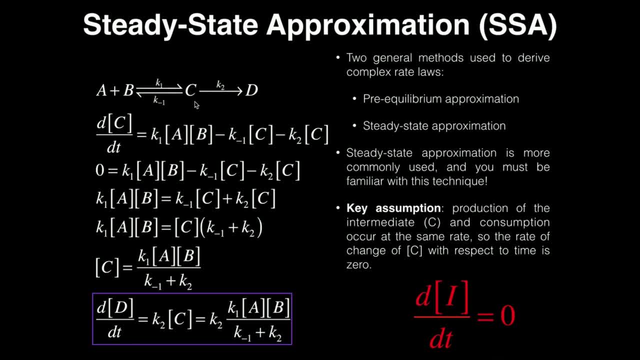 equal to the rate of the consumption of C. So whatever C is being formed, it's immediately consumed at the same rate to form the product D. What that means is that, even though I always have some concentration of C, because some is being formed, 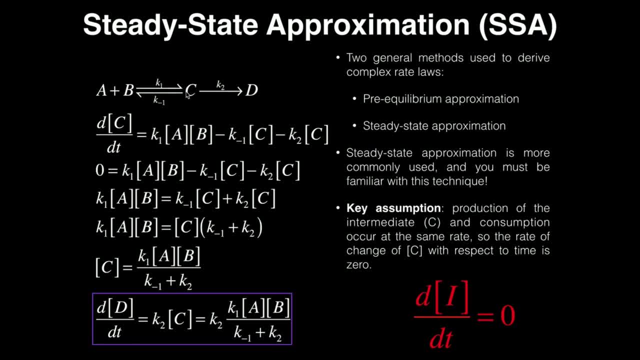 the rate of change of the intermediate with respect to time is zero, meaning this concentration of C is not changing with time. That's a key assumption. So what we say is this: general derivative right here, the rate of change of the intermediate with respect to time is zero- or the derivative of the. 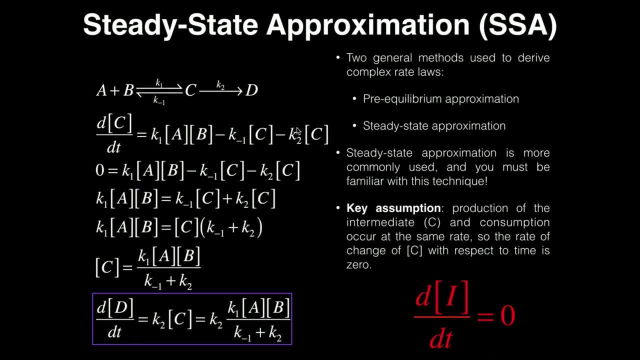 concentration of the intermediate with respect to time is zero. Now, in the context of this equation, C is my intermediate, so I could put a C right here and say DC to DT. All right, let's look at the equation up here at the top I 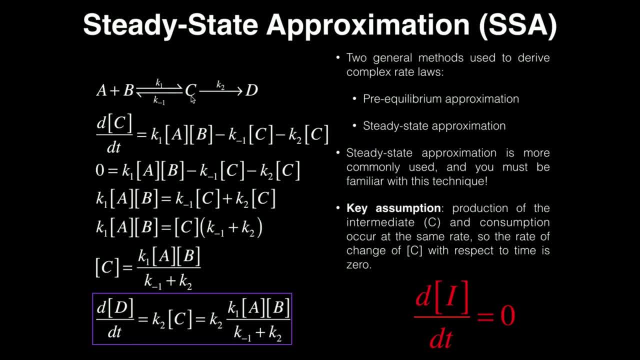 have two reactants: A and B are in equilibrium with species C, and the forward reaction is given by K1, the reverse reaction is given by K-1, and then C can be consumed to form the product D. in relation to this rate. 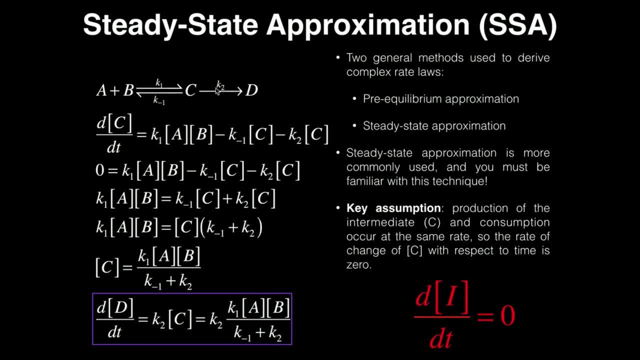 constant K2, right? So in this equation, C is what we call an intermediate. okay, it is both formed by this K1 reaction, but also consumed by a C, by the K2 reaction. So it's both formed and consumed, which makes it an intermediate. Now in 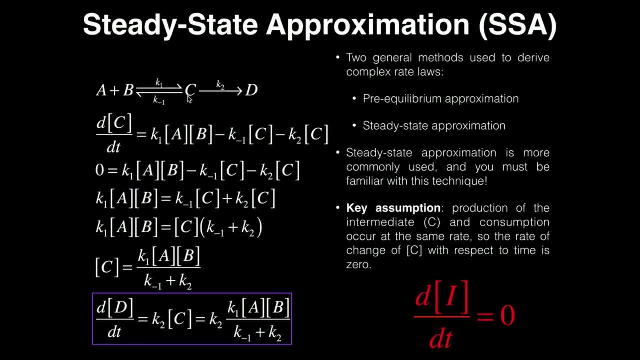 the steady state approximation, we have a very important key assumption, and that is that the rate of formation of C is equal to the rate of consumption of C. That basically means in layman's terms, whatever C is formed, it's immediately consumed to form D. So the rate that C is being 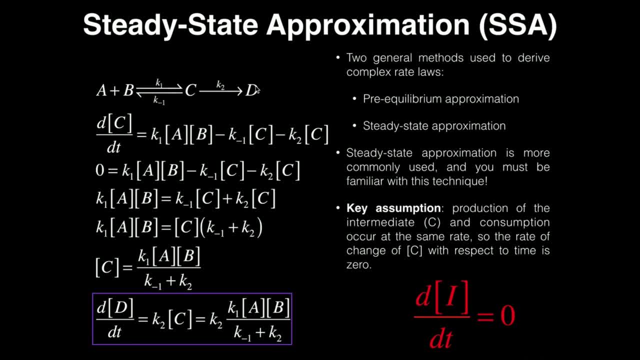 made is equal to the rate at which it's being consumed, And so what that means is that the rate of C with respect to T, in other words the change in the concentration of the intermediate C with respect to time, is zero, because any C that's formed is consumed at the same rate. So there is 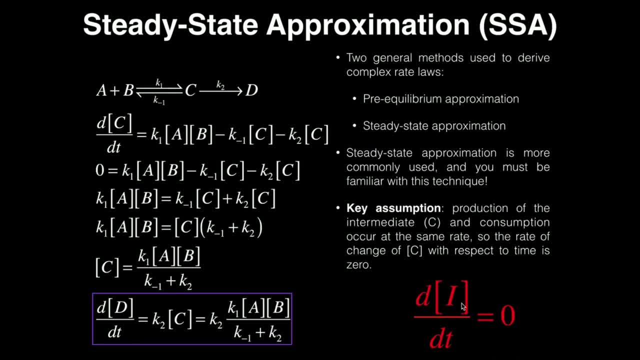 an actual non-zero concentration of the intermediate C. it's just that its rate of change with respect to time is zero, because any that's formed is consumed at the same rate, And this is the general derivative that expresses that, and this is the key assumption right here. 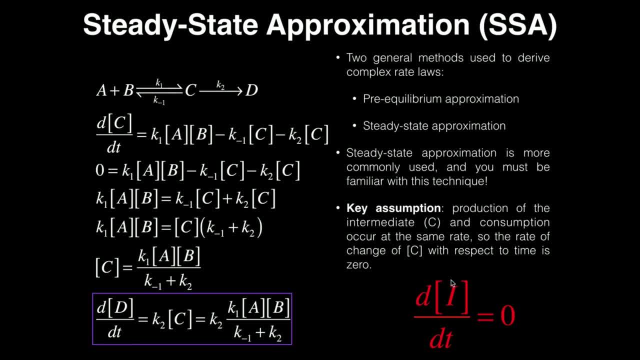 And in the context of this equation, we could replace this intermediate I with C and say the derivative of the concentration of C with respect to time is zero. or I'll just say dC. dt equals zero. Now, whenever you do a steady state approximation problem, every single time, you always start with: 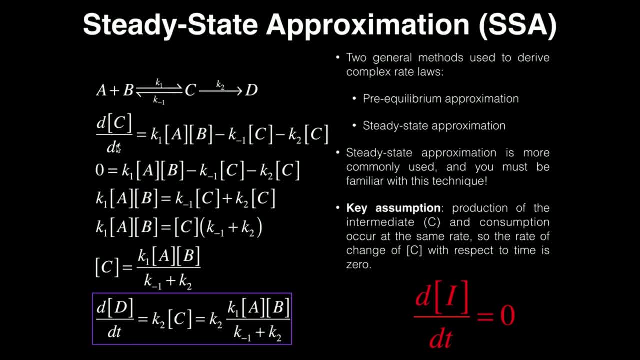 whatever the intermediate is, and you look at its change in concentration with respect to time. If the intermediate in some other one was dF, you would start with dF, dt. Now we want to set up an expression for how the concentration of that intermediate 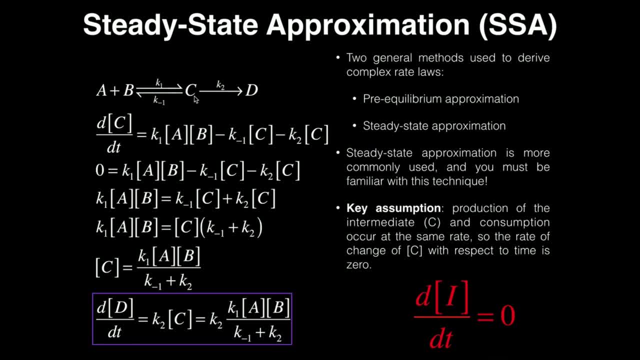 changes with time. So let's look at what forms C. The only reaction that's forming C is that of K1, so it's going to be positive K1 times its reactants a인B. Now we have two reactions that are consuming C, so decreasing its concentration. 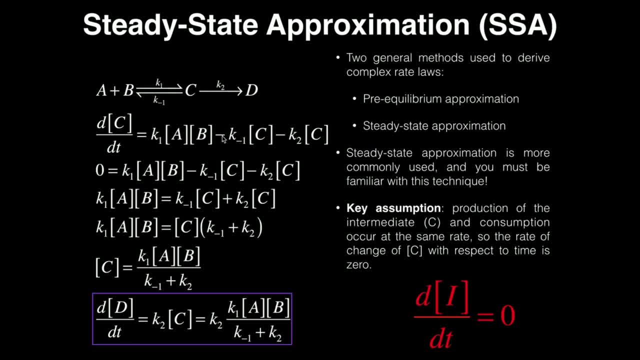 and K2.. Well, the reason this 1 is negative is because it's removing C effectively, because it's going backwards. So the rate would be K-1 and the substrate with respect to that reaction is C, because we're moving to the left. Okay, so it'd be K-1, C with a minus sign, and then this other reaction is going to. 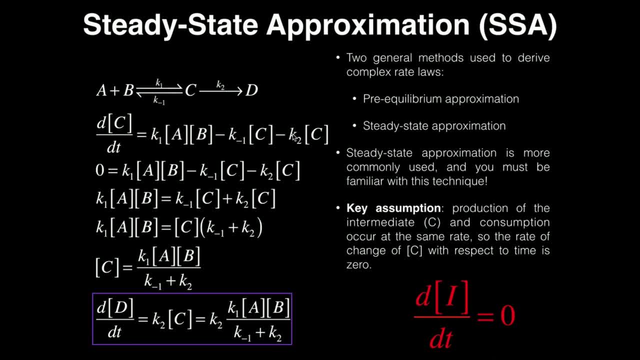 the right. it's also consuming C. So we have K2, its rate constant, it's a negative and then times the reactant of that particular reaction, C. So that is my expression for how the rate, how the concentration of C, the intermediate, changes with time. But I can set this derivative equal to zero. 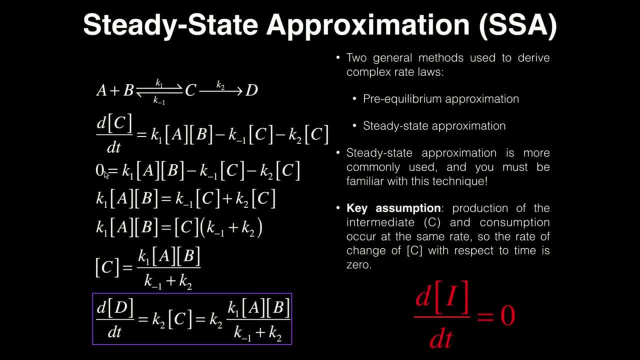 because that's our key assumption of the steady state approximation. So I set it equal to zero and then what I'm going to do is I'm going to solve for the concentration of whatever that intermediate is. Okay, so solve for, in this case, C. So what I'm going to do is I'm going to move. 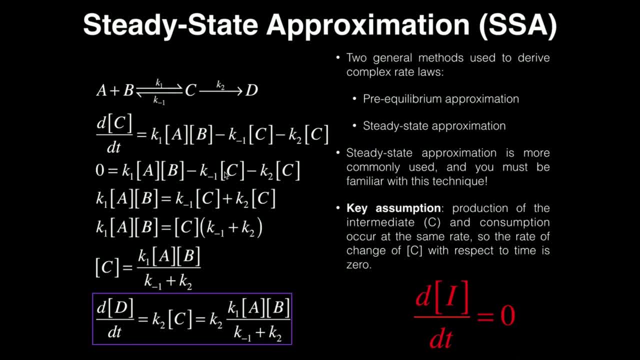 all of these, the negative expressions, because they all contain a C over to the other side. Okay, so what I'm going to get is a positive K-1 times C plus K2 times C. On the other side, I still have K1 and then A. 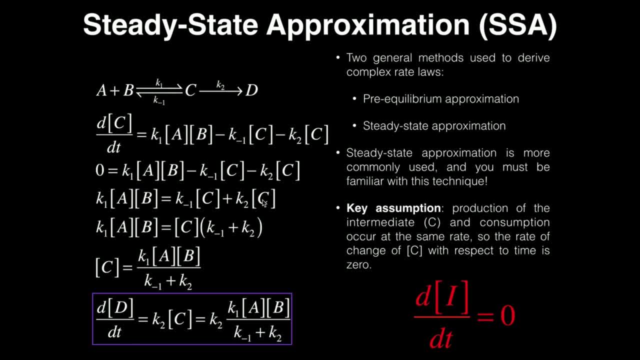 times B. Now all my C's are on the other side. So I can factor out that concentration of C and what I get is K-1 plus K2 equals K1 times A times B. Now I can get an expression for the concentration of C by dividing both sides by the sum K minus 1. 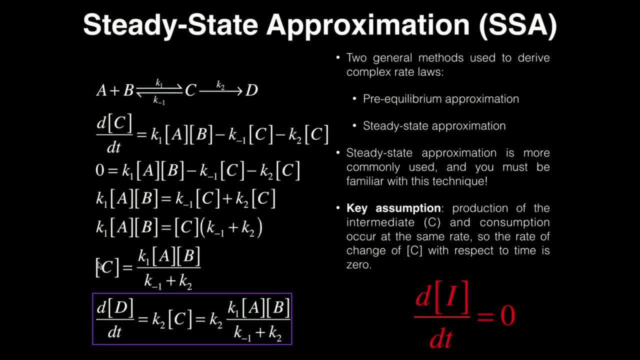 plus K2.. So that means my concentration of C is going to be equal to K1 times A times B, divided by the quantity K minus 1 plus K2.. Now how is that useful? Well, I want the overall rate of this equation, which is described by this last reaction right here, C goes to D in relation to K2.. So what? 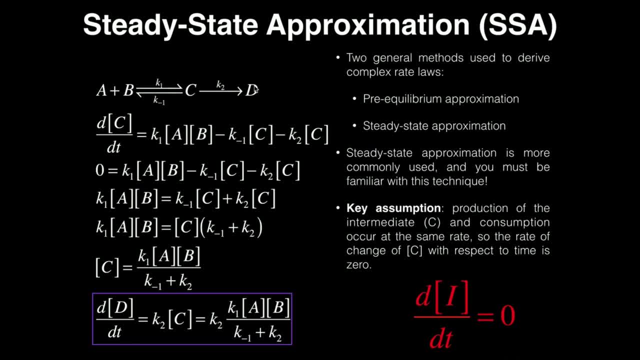 is the rate of this equation? Well, I want the rate of this equation which is described by this last. So, what is the rate of this equation? Well, I want the rate of this equation, which is described by this: the formation of D. How do I express that rate? The formation of D is the change in concentration. 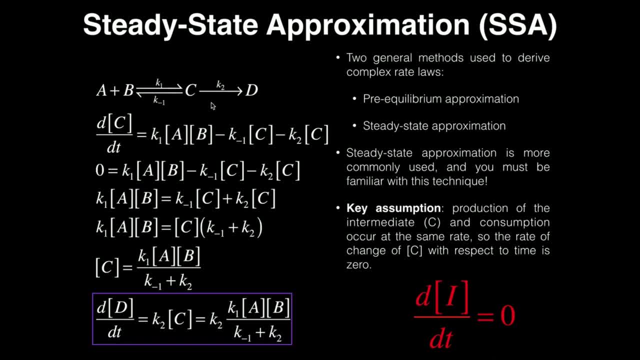 of my product, D with respect to time, is equal to its reaction K2 times the reactant or substrate concentration of C. Well, that's pretty handy, because I just calculated what the concentration of C is equal to in other terms, So I'm just going to plug this entire expression in for.